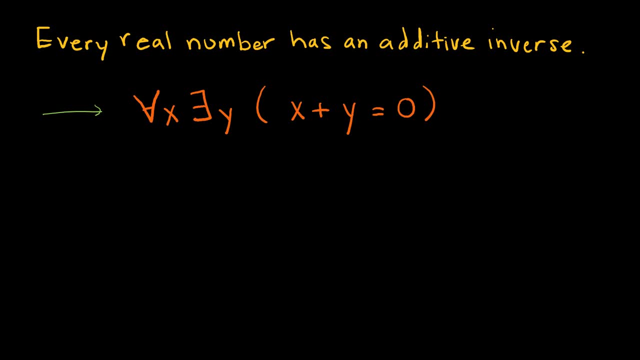 there exists a y, such that x plus y equals zero. For now, however, I just want to discuss: when is this true? or is this true, or how do I know? what is the process involved? So we can see here that we have a domain. 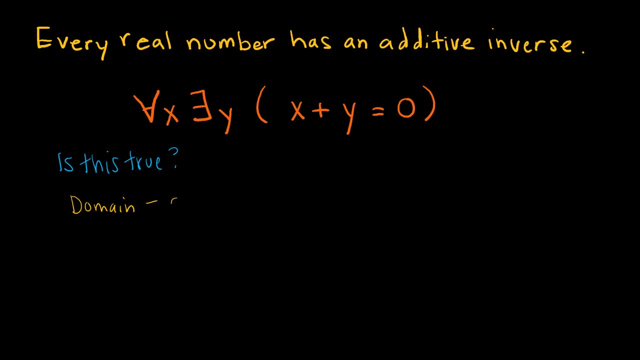 of all real numbers, every real number. So, in this domain, because it's all real numbers, in order to show that this is true, we would have to use real numbers. So, in this domain, because it's all real numbers, we would have to use reasoning and proof, because we can't go through an exhaustive list of all the. 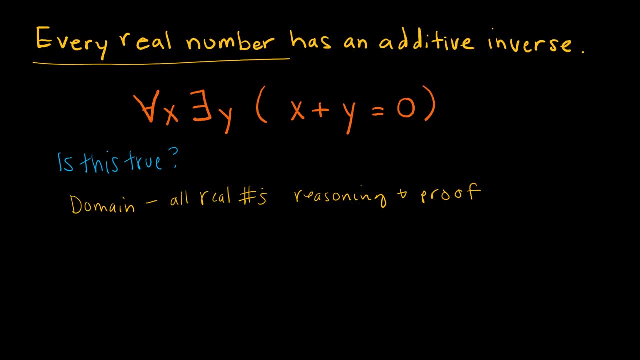 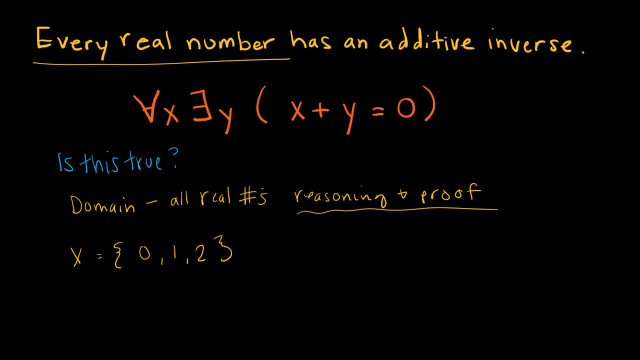 Now this is a completely different scenario, because what I have is: I have a list of values And what I can do instead is, again, we're still going to assume y is just any real number. So now what I'm saying for all x in my set of numbers. 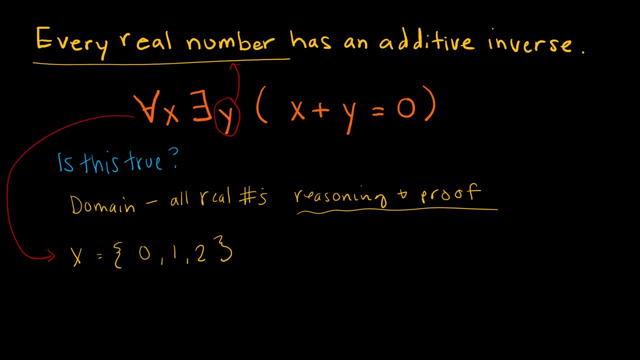 there exists some y that is a real number, such that x plus y equals zero. Or I'm saying zero plus blank equals zero, Zero plus sorry- one plus blank equals zero And two plus blank equals zero. And if I can find a value to replace to make that statement true, and those values all. 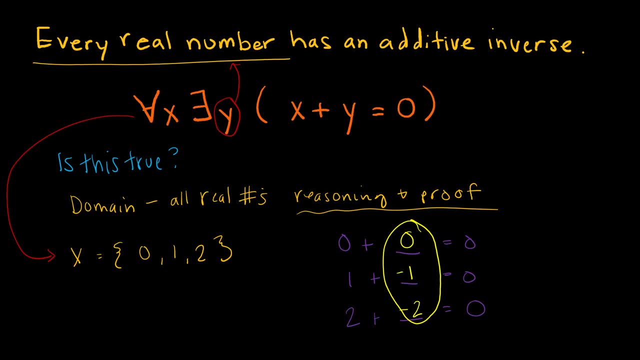 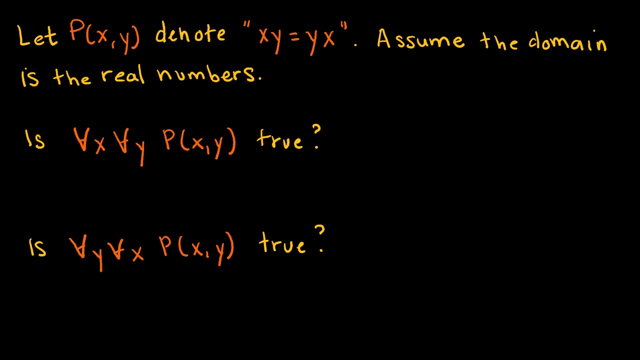 belong to the real numbers, which they do, then essentially I have proven it's true. So I've cycled through each of these numbers and shown that it is true. So let's take a look at this example. We're going to let p of xy denote that x times y equals y times. 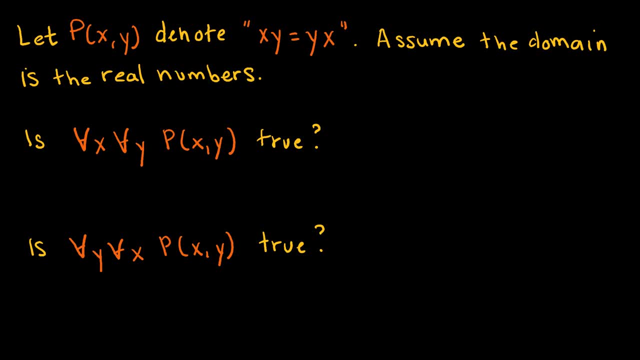 x, We'll assume that the domain is real numbers. So I have two different statements here, And before we talk about whether they are true, I want to talk about what I notice about them, And that is here I have for all x and for all y. Here I have for all y and for all x. 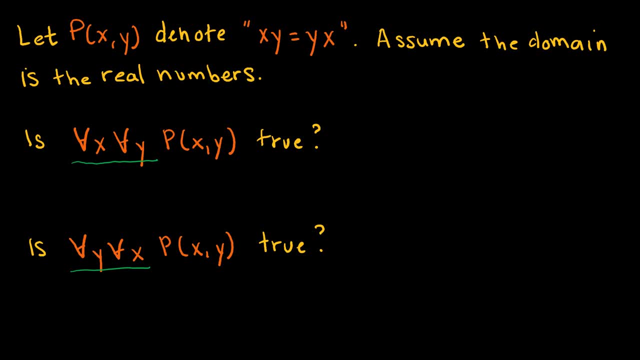 So essentially what I'm asking is: first of all, is this statement true? And then I'm saying: is it still true if I change the order of x and y? So what exactly does our statement mean? This first statement says: for all real numbers x and for all real numbers y. 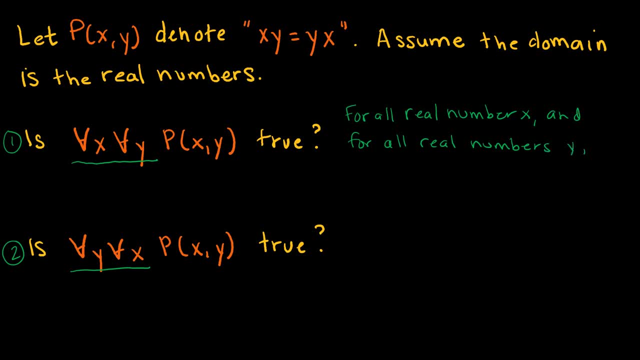 the order is true if plus or minus x times y equals y times x, So would that not mean, after all, are all x times y equal x? Or if it's x times y is equal x times y. So what about x or y? 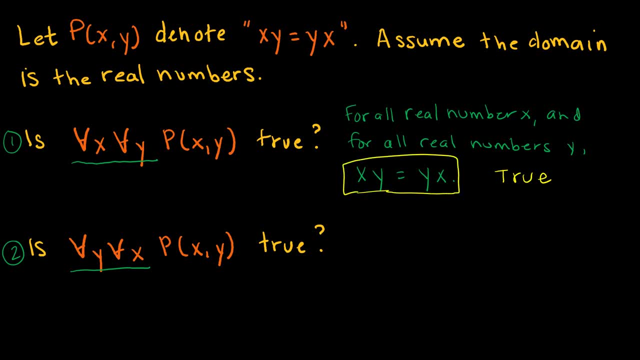 equals x times x. Well, I saw in my structures痠 they're being used like cannot be considered objective because they're always the same property. I have to remember that the order is the property of multiplication. a property can or can't be considered objective enough because nn means that I havestopping, that nn equals loading room. 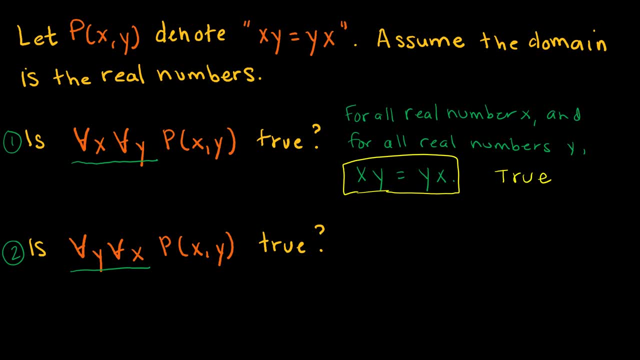 So it's x times y'll end up at the same product. I've shown that the first one is true, not through a formal proof. but number two says: is for all y and for all x. so essentially it means this exact same thing. but now I'm. 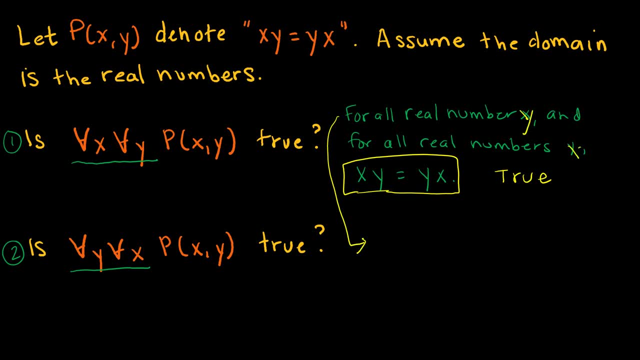 saying: for all real numbers y and for all real numbers x. is that statement still true? And yes, in fact it is, because, as we had said before, the order doesn't matter. So in this one, both of these statements are true. 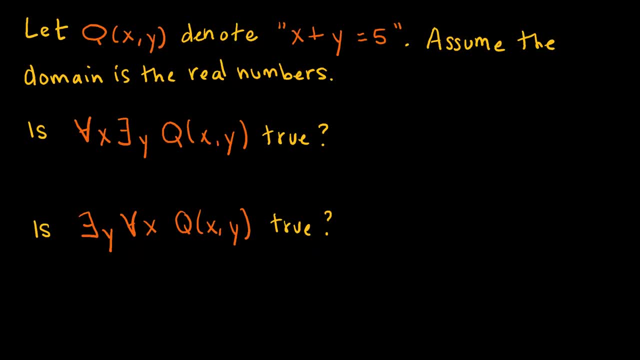 It didn't matter if x came first or y came first. Now let's take a look at a different example. It says: let qxy denote: x plus y equals 5.. Again, the domain is all real numbers. So let's start with our first statement. and our first statement says: is it true that? 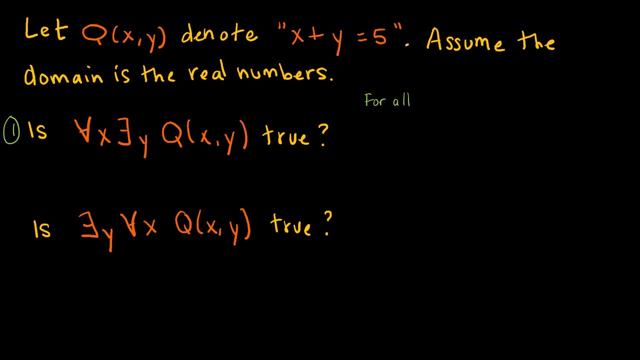 for all real numbers, x, there exists a real number, y, such that x plus y equals 5.. So the question is: is this a true statement? So it's really important here to understand the for all and there exists. So this is saying: for every single real number, does there exist some other number? 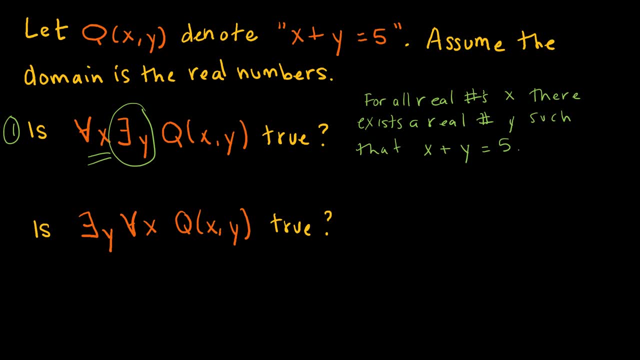 Such that when we add them together, we end up with 5.. And of course, this statement is going to be true Because for all real numbers, for instance 2.. What number could I add to 2 to get 5?? 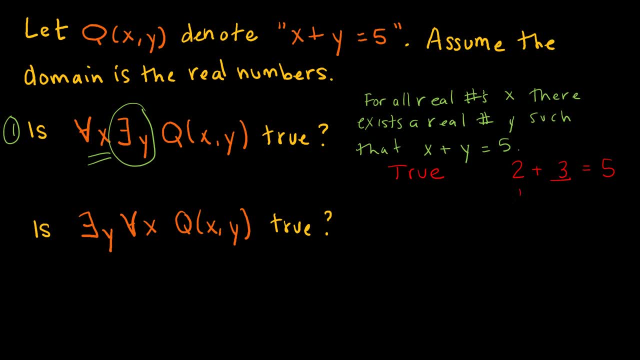 3. So what about 1 half, 1 half plus what equals 5?? Again, we're dealing with any of the real numbers. So 1 half plus 4 1⁄2. Or 9 halves would equal 5.. 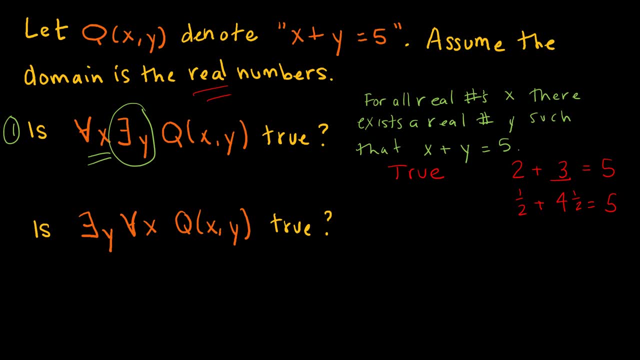 So that is always going to be true. Now my second statement is a little bit different. Is: there exists a y, So there exists a real number, y, Such that, for all real numbers, x plus y equals 5.. So some might say: well, that is the exact same thing that we just did in number 1.. 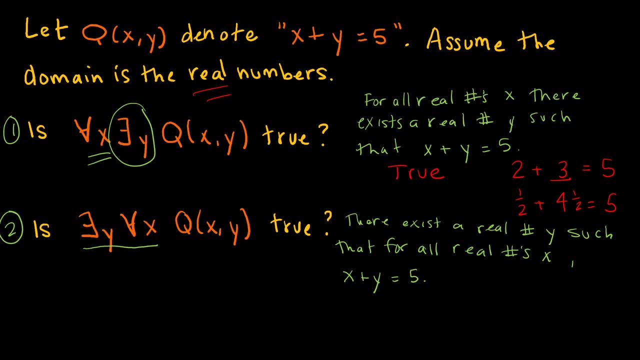 And that is unfortunately not the case here. We're saying: there exists some real number, such that for all real numbers, x, x plus y equals 5.. So we're saying: is there 1 number, y, just 1 number, it can't change based on each case, such that for all real 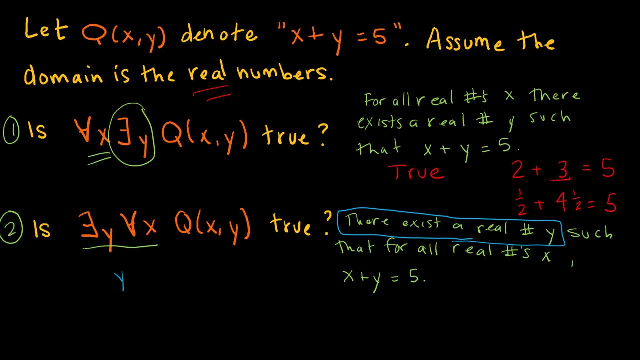 numbers x. x plus y equals 5.. So let's let y equal 0.. Well, if x is 1, then I have: 1 plus 0 equals 5, and that is not true. So the only time that would work is if y is 4.. 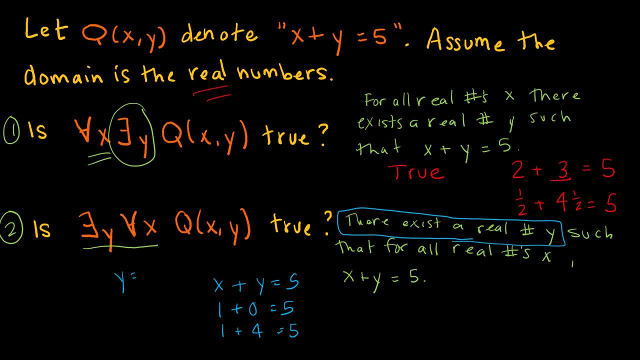 Okay, so for the sake of argument, let's let y equal 4.. Well then, let's say x equals 2, well then I get: 2 plus 0 doesn't equal 5,, 2 plus 4 doesn't equal 5.. 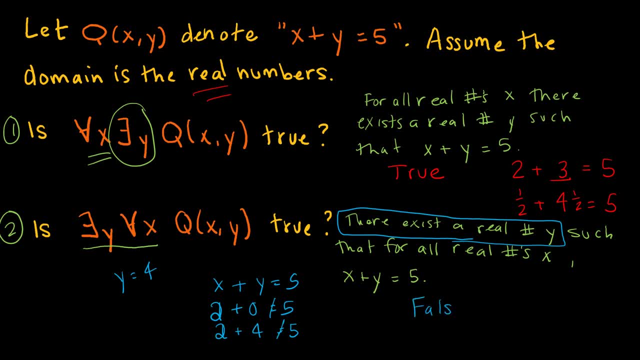 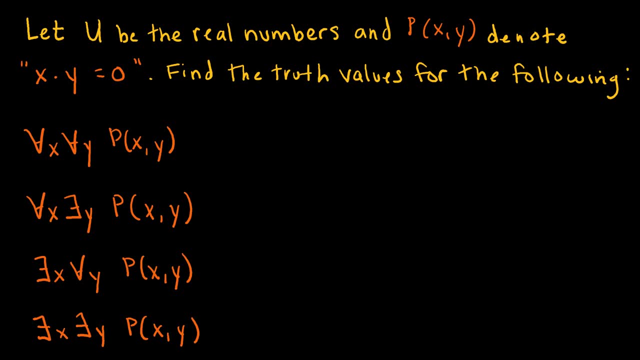 So we can see that the second statement is false. Let's take a look at a couple of practice together. Here we have: u is the real numbers, so the domain is all real numbers. p, x, y denotes x times y equals 0.. 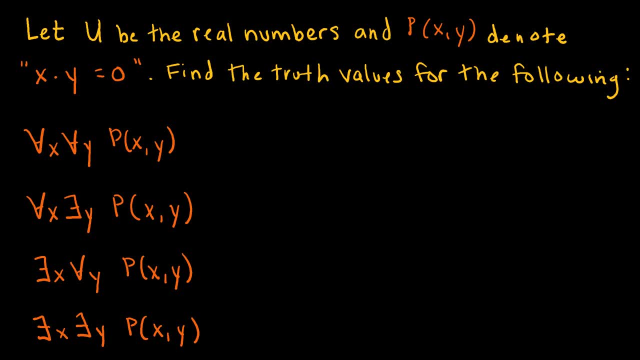 And we're given several different propositions here to find the truth- values for. So we'll start with the first one: for all x and for all y. So for all x, then for all y, p, x, y is true. So essentially they're saying: for any real number x and any real number y, x times y. 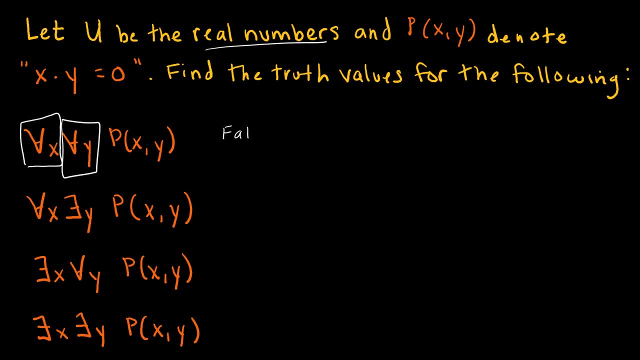 equals 0.. It's pretty easy to determine fairly quickly that this is false, And remember: to show something's false, all I have to do is show a counterexample. So 2 times 3 equals 0, obviously not true. 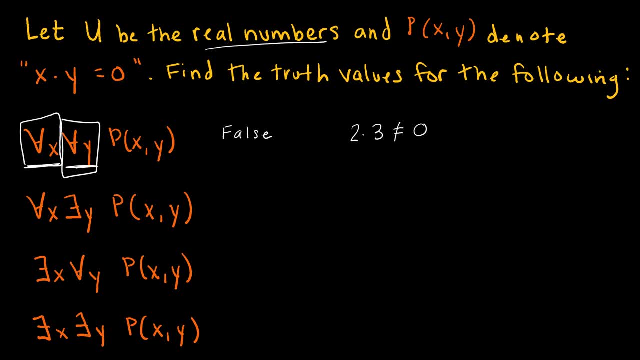 This is a counterexample, because for all x and for all y tells me, I can choose any x I want and any y I want, and x times y would be equal to 0. So again, that is in fact false. Let's look at the next one. 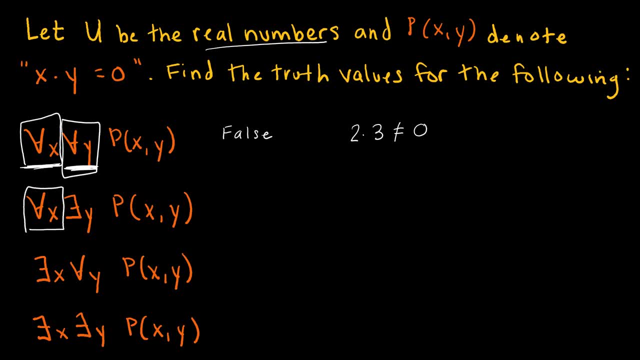 For all x, so for any x I can think of, there exists some y such that x times y equals 0. So for any x I can think of, say 13. Can I think of a number that would give me a product of 0?? 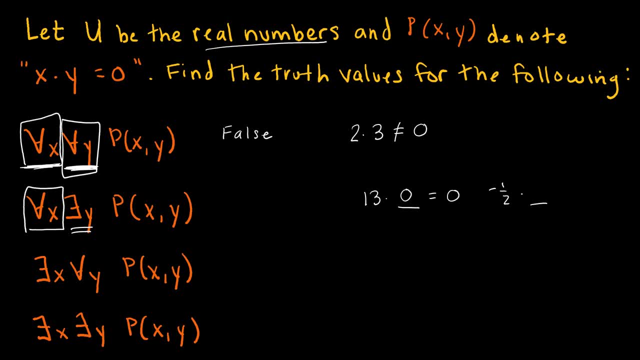 Yes, What about negative 1 half? Can I multiply by something to get 0?? Yes, Now, in this example, that space, that thing, that y that exists, happens to be the same value. That's not necessary. It is necessary in this case because, obviously, if we take something times 0, we get 0. 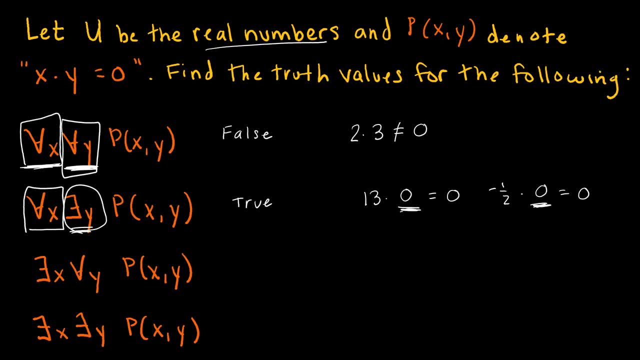 But it's not necessary for the quantifiers. Let's look at the next one. There exists some x for all. y p of x is true, So this one can get a little bit tricky. Now, this one is still going to be true, but I want you to pay attention to this in our 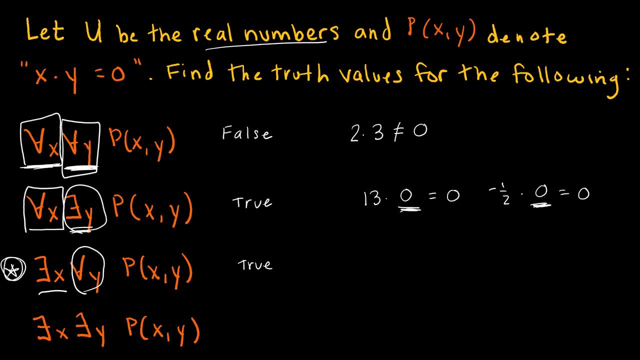 next example, Okay, little bit different. So again, this one's going to be true because it says there exists some x that for all of y. this is true. So there exists some x such that for any y, for all y's. so 2 and 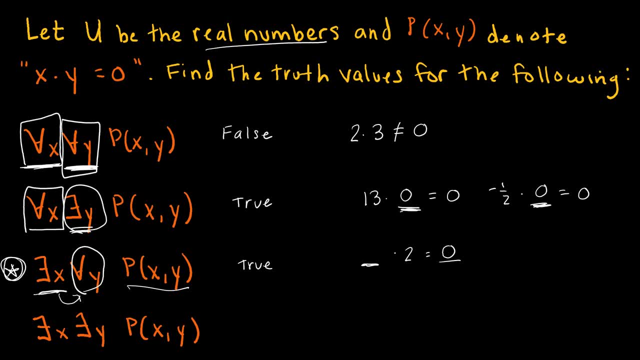 4 and 19 and negative 37, that I'm going to get a 0. Now, in this case, yes, I'm still going to be using 0 as that space. but this one's tricky because this one happens to be true, because 0 times anything is 0. But if my statement up here were a little bit different, 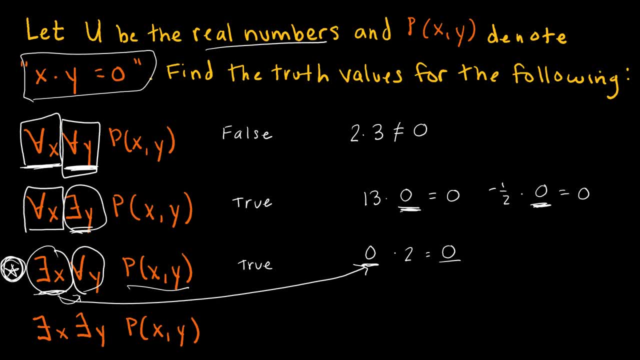 this quite often will be a false statement, because this is saying there exists one x, such that it is true for all y's. So hopefully that'll make more sense when we do our next example And then for our last one. there exists some x and there exists some y, and of course we know that. 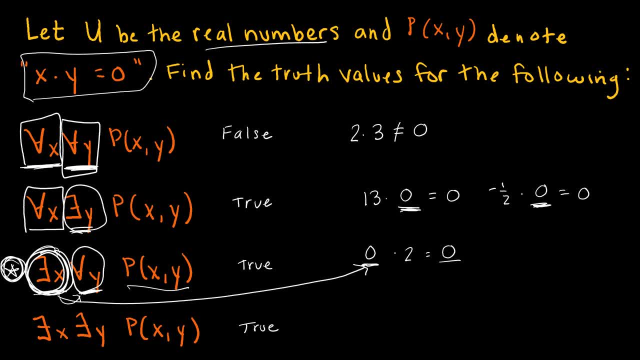 this is true. That's saying, I can find an example that shows that this is true, and obviously we've already shown several examples. Negative 37 times 0 equals 0.. 0 times negative: 4 thirds equals 0.. We get the idea that all you'd have to do for there exists is just show one example. 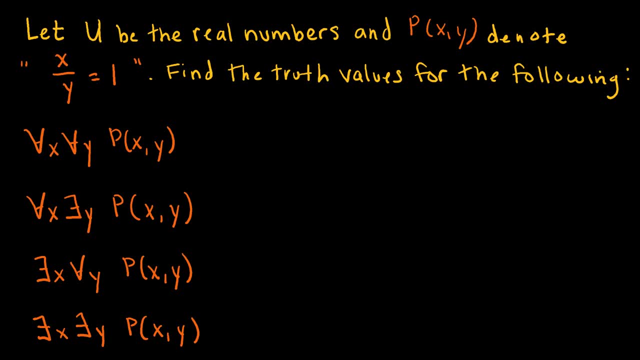 Here's one for you to try. So, if you'd like, you can go ahead and press pause on this video and try these questions for yourself first, and then we're going to go over them. So, when you're ready, press play to see how you did So. this is a very similar question, except for now, instead of addition, we're 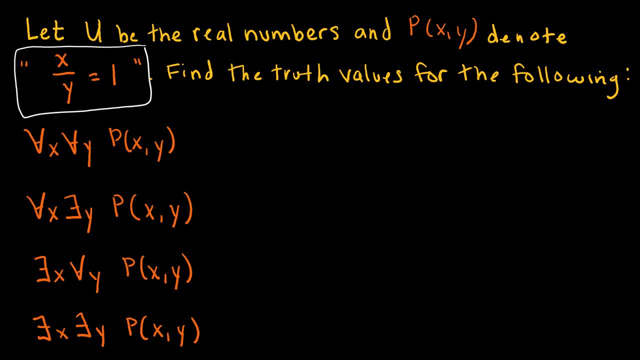 dealing with division and it says: use the universe of real numbers. pxy denotes x divided by y equals 1. find the truth values. So again the first one, pretty straightforward. We're saying: for all x's and all y's, when we divide them we get 1.. Well, obviously this is false and 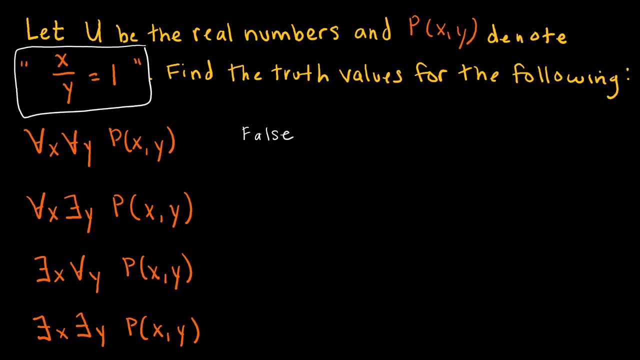 all I have to do to show that it's false is to show a counterexample. So 10 divided by 2 equals 1 is in fact not true. So that's false because it doesn't work all of the time. The next one says: 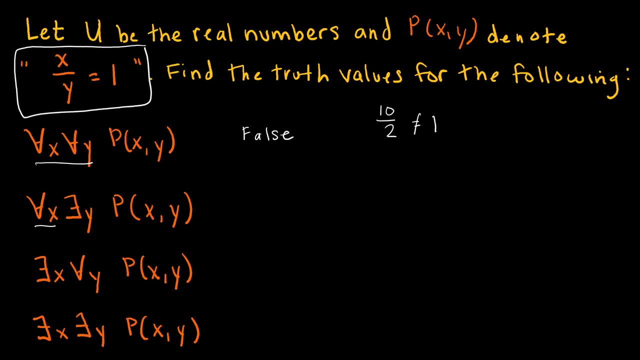 for all x, there exists some y, such that this is true. Now, this one actually is false, and we want to say that it's true, but it's false because we're dealing with real numbers, and so, even though I'm going to show you the one case in which this is not true, 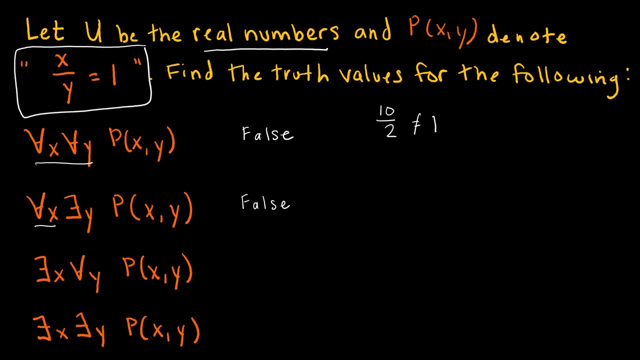 So normally we could say, for all x, for any x that I can think of, say 18, there exists some y and this y can change, so there's some number that I can divide to get 1.. And of course we would say: 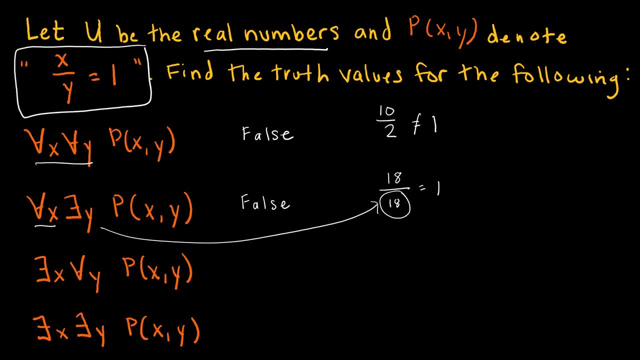 yes, that's true, Because if x is 18, just make y 18.. And if x is negative 32, just make y negative 32.. And when I divide those, I get 1. And I would say you're correct. However, because we're saying: 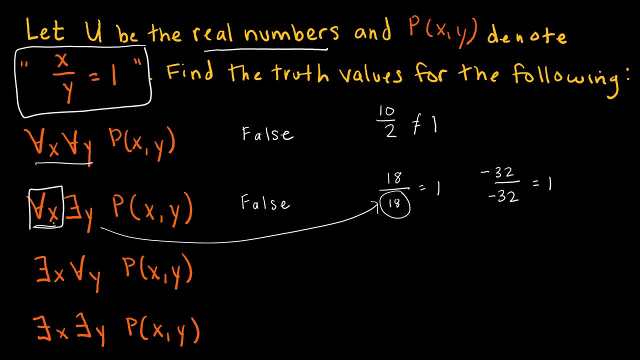 for all x's, for every value of x. that is a real number. we can find some number such that when I divide, I get 1, unfortunately is false, Because I'm going to move this guy out of the way- because one of the real numbers is 0. And 0 divided by anything I can think of for y: 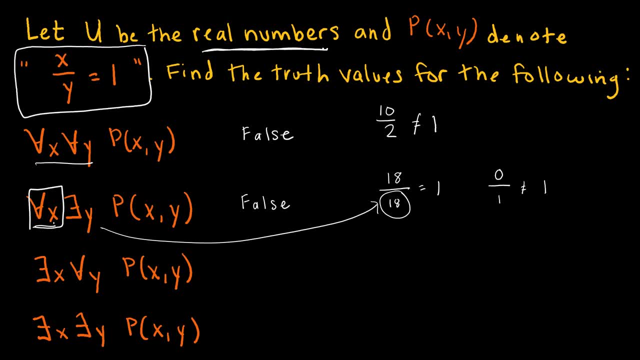 is never, ever going to give me 1.. So, even though it works all of the time, except for when x is 0, unfortunately that makes it false, because I can provide a counterexample. So let's look at the next one. There exists some x such that for all y, this is true. 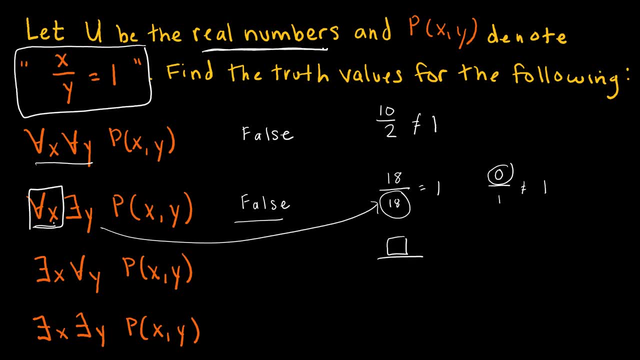 So we're saying x has to be just one value, such that when I choose a y, any y that I want, that I'm going to get 1.. Well, this, unfortunately, is going to be false as well, Because there exists some x, such that this is true tells me that it's just one x value. So say, x is 15.. Well, that's going to work when y is 15.. But if x is 15 and y is 32, that doesn't work anymore. 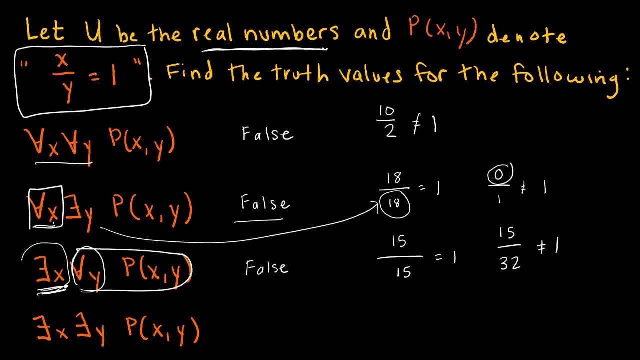 So this one is false because we're essentially saying we can fix some x value such that it's true for all y values. And of course that is false For the last one. there exists some x and some y, such that it's true. And obviously this is true because we can show 13 divided by 13 is 1. And that's all we need to do for there exists is show that it is possible. 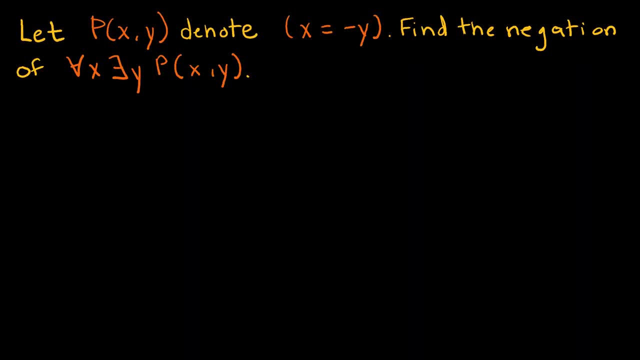 And for our last question together: in this video let p, x, y denote that x is equal to negative y And we want to find the negation of this statement. So this is the first time we're doing a negation of a quantified statement. When we negate a quantified statement, essentially what we're trying to do is we want no negation. 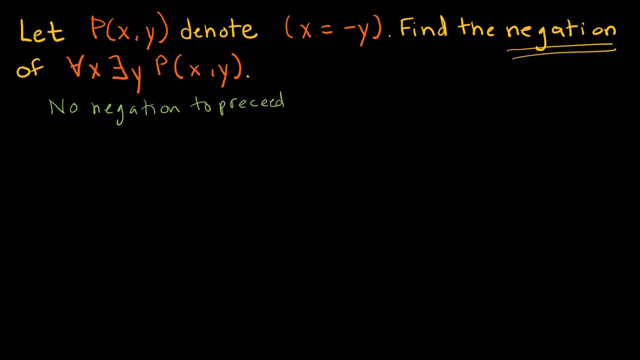 to precede a quantifier. So what I'm being asked to do is I'm being asked to find the negation of for all x, there exists a y, such that p x, y, And what I need to do is think about how am I going to? I'm going to make this one a quantifier. 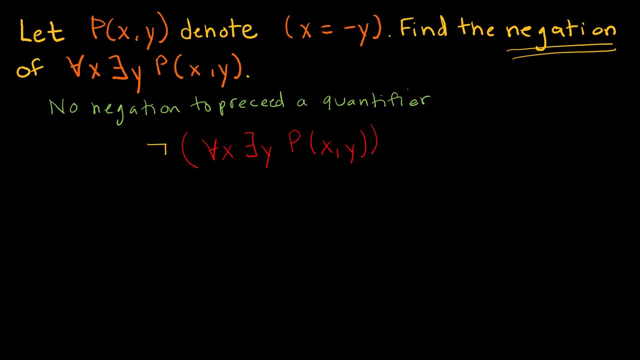 different color. how am I going to negate this? so we talked about negating quantifiers and a few videos ago, and what we're going to do is, essentially, we're going to just start by taking the negation that was a bad one, the negation of for all X, which, of course, the negation of for all X gives me there.